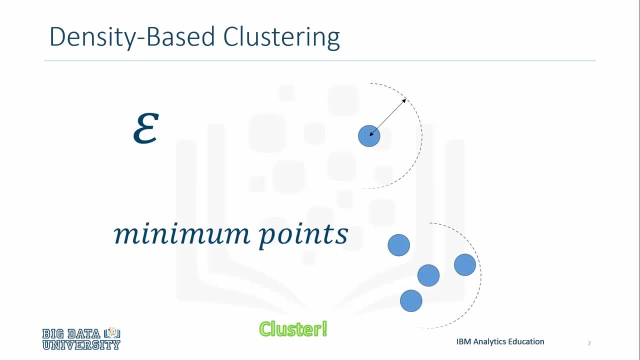 account epsilon and minimum points. Epsilon is the maximum radius of the neighborhood and minimum points is the minimum number of points in the epsilon neighborhood to define a cluster. There are three classifications of points. They are core, border and outlier. A core point has at least minimum points within. 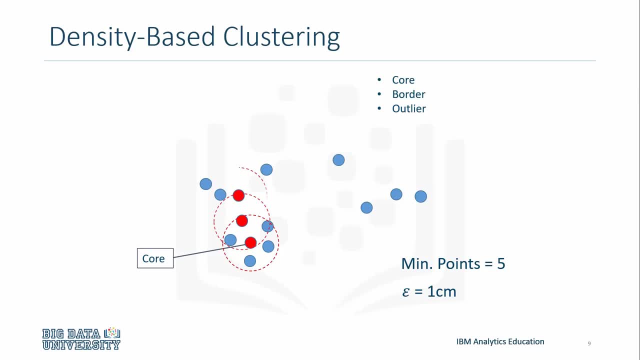 its epsilon neighborhood. These are points that are at the interior of a cluster. A border point has less than minimum points within its epsilon neighborhood but can be reached by the cluster, That is, it's in the neighborhood of a core point. And finally, an outlier or Vorikids' noise point is a point that cannot be reached by. 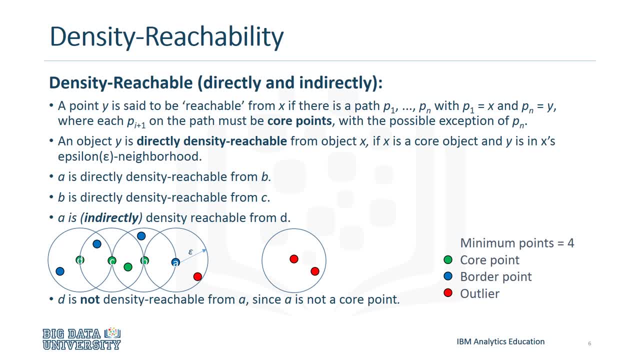 a cluster, A point y is said to be reachable from x. Ifaster is fixed to e, P1 to Pn, with P1 equals x and Pn equals y, where each Pi plus one on the path must be core points, with the possible exception of Pn. 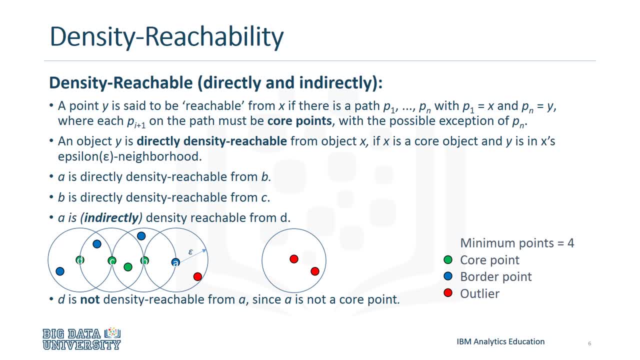 An object, y is directly density reachable from object x. if x is a core object and y is in x's epsilon neighborhood, A is directly density reachable from B. B is directly density reachable from C. A is indirectly density reachable from D. D is not density reachable from A, since A is not. 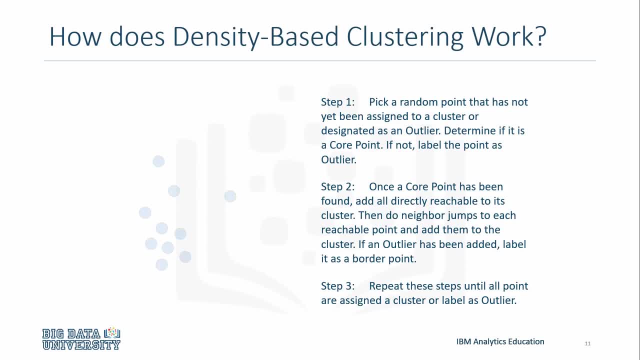 a core point. Density-based clustering works by picking a random point that does not belong to a cluster or is an outlier and determines if that point is a core point. If not, you can label it as an outlier. Now we'll pick another core point at random and determine if it is a core point. 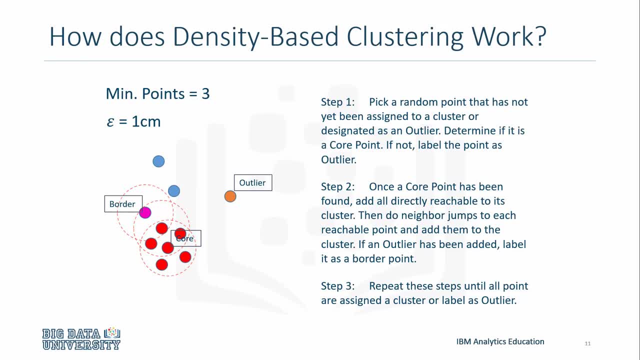 If it is a core point, then all of the directly reachable nodes are assigned to the cluster. Then do neighbor jumps to all reachable points and add them to the cluster. Keep finding neighbors until you're unable to. This point would be labeled as a border.